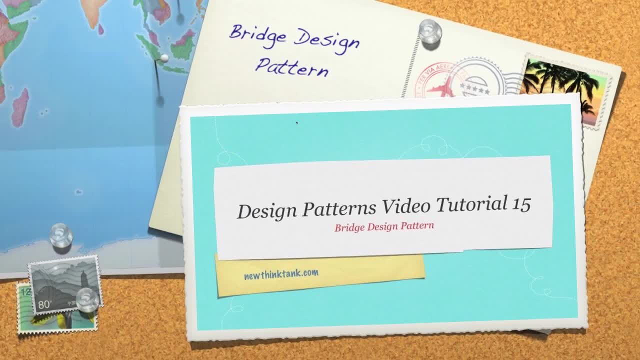 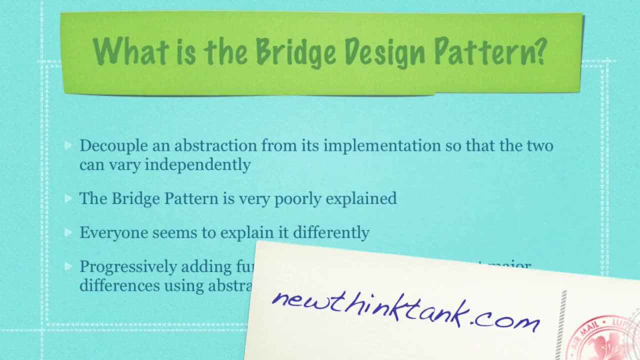 Hello internet and welcome to part 15 of my design patterns video tutorial. Today I'm going to talk about the bridge design pattern. So what is the bridge design pattern? Well, the official definition is to decouple an abstraction from its implementation, so the two can vary independently. 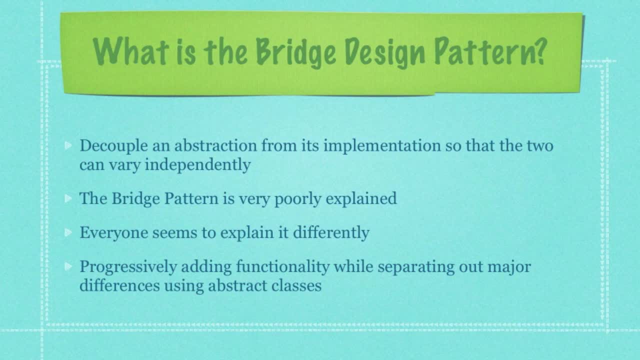 Yes, that is a bunch of gobbledygook, and I have found through numerous different tutorials that the bridge pattern is often very poorly explained or glossed over completely, and on top of that, everyone seems to explain it differently. In this part of the presentation, I'm going to explain it. 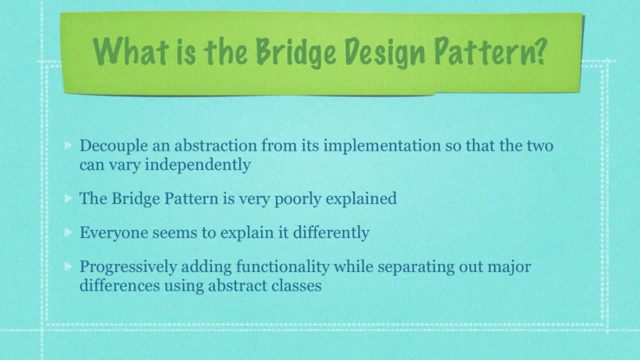 the way that I have always used the bridge design pattern and the way that it was explained to me by someone much more intelligent than I, And my basic definition is to progressively add functionality while separating out major differences using abstract classes. So let's go into a bunch of 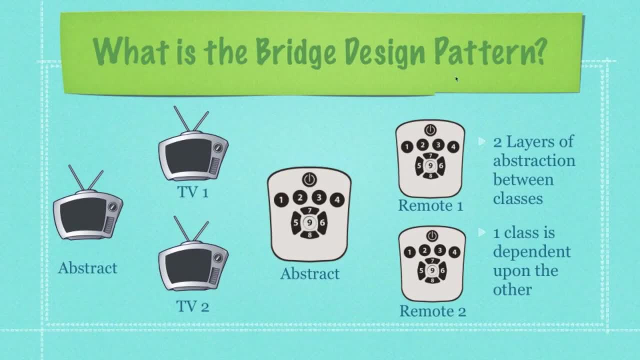 pictures and explain this further. So let's say that you want to come in here and you want to ultimately create remote controls that are going to work differently depending upon very specific conditions. So let's say that you want to come in here and you want to ultimately create. 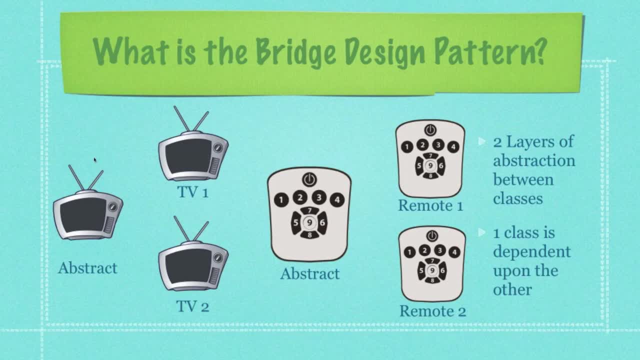 specific televisions and, along the way, you want to define all of those attributes that each television or device will have, and then remote controls along with that. So if you're going to be creating the most abstract of televisions, what are two bits of functionality that every 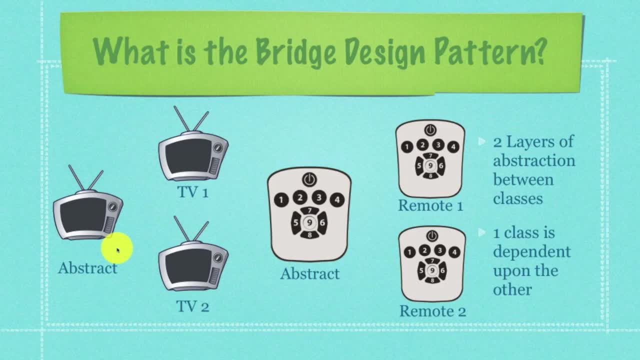 single device ever is going to have. Actually, in fact, whether it's a television or a radio or a DVD or so on, each one of them is going to have a remote control that is going to control volume. So what we're going to define here, 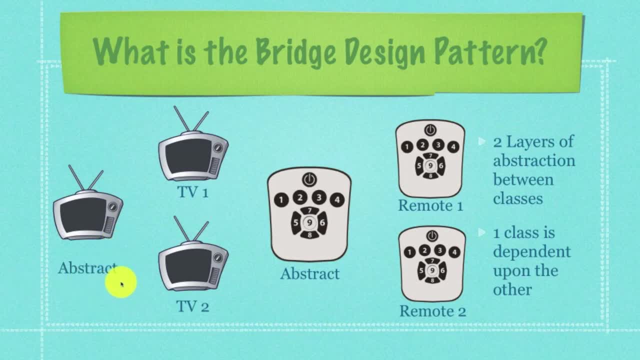 in our first abstract class are the buttons that are going to define volume for all of our devices. Seven is going to represent up volume and eight is going to represent down volume. Then afterwards we're going to create more concrete devices and this first television, which we're really going to. 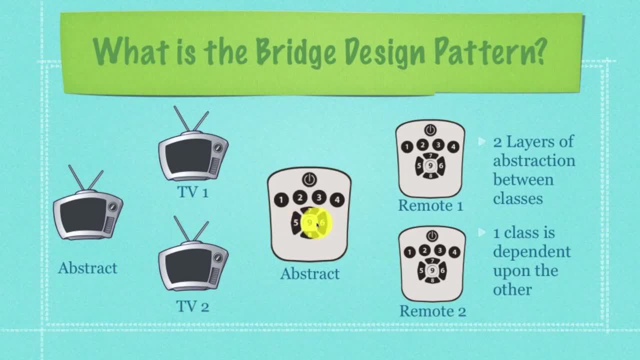 focus on is going to define what five and six are going to do, Which means they're going to define that the channel number should increase whenever six is pressed or decrease whenever five is pressed. However, let's say TV two is actually a DVD player. In that situation, button six will skip to the next. 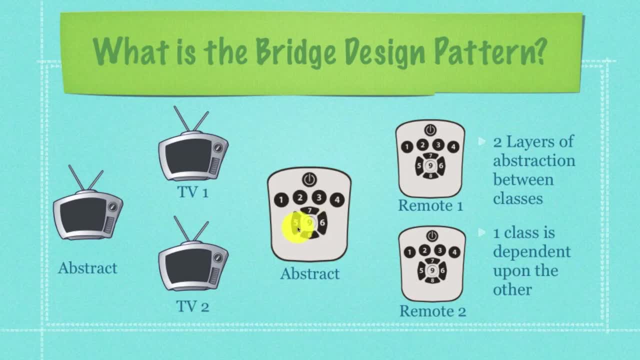 chapter, while button five will skip to the last chapter. Then we come to our abstract remote control. What it is going to hold is a reference to a specific device, either the basic TV or the TV that is going to have a DVD player connected to it. It is then going to define all those abstract. 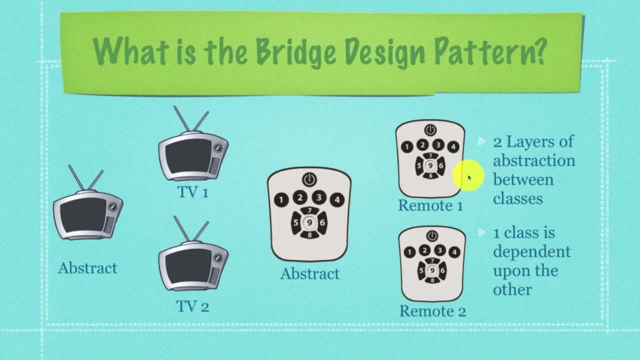 methods that are going to differ between this remote right here and the device that is connected to it. This remote right here and those very specific differences are going to lie with button nine. Remote one, whenever the button nine is pressed, is going to mute the sound, while down here with 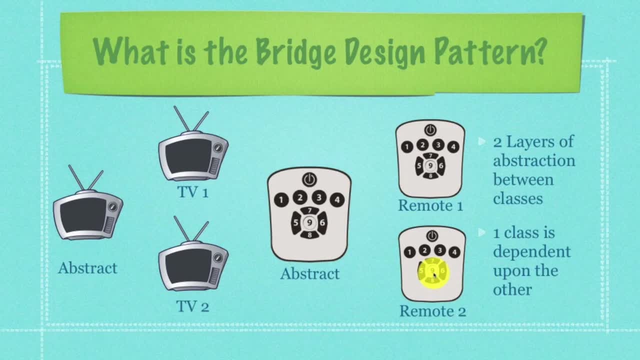 remote two that we're going to define. whatever it is pressed, Let's just say it's going to be connected to a DVR which is going to pause the television. So, along the lines, we're adding different layers of functionality, with an abstract class that lies between Hence, two layers of 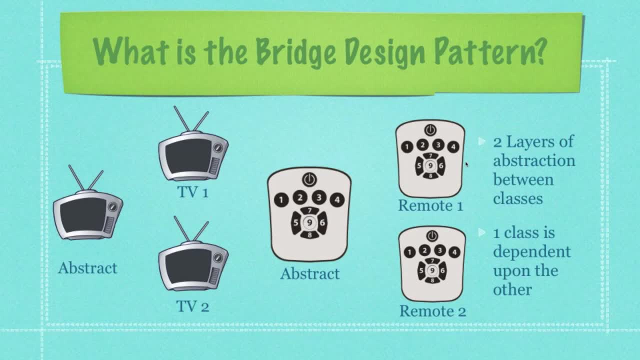 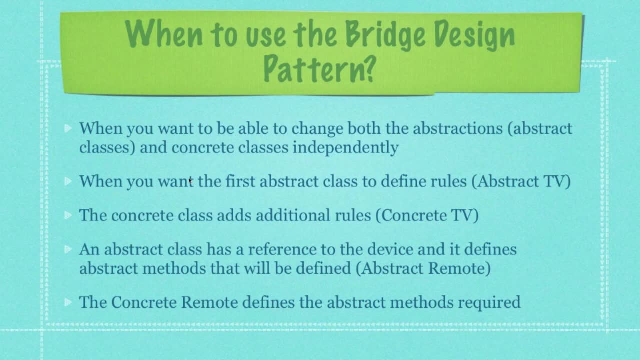 abstraction between classes and one class that is going to be dependent on the device. So when should you use the bridge design pattern? When you want to be able to change both the abstractions or the abstract classes along with the concrete classes completely independently. So, like I've showed previously, when you want to have your first abstract class defined certain. 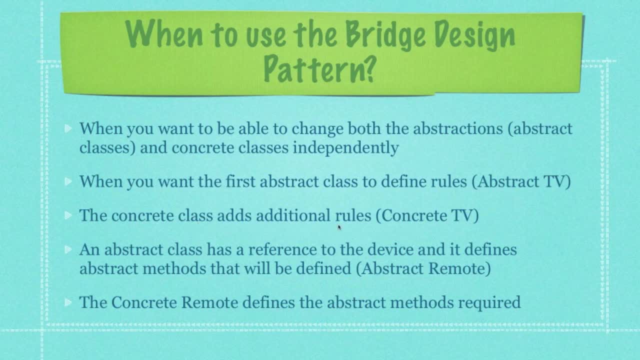 roles and then create a concrete class that adds additional roles for the concrete televisions, And then you're going to have another abstract class that's going to have a reference to each one of these devices and it's going to define all those abstract classes that are going to be. 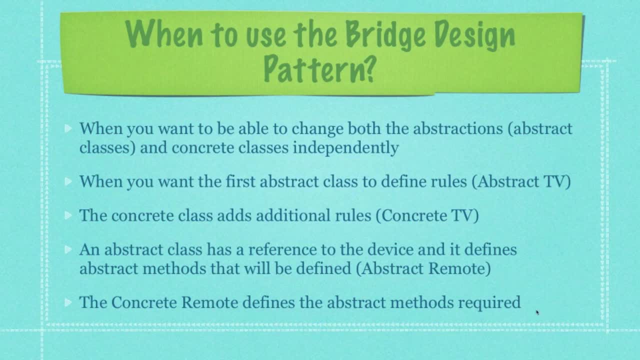 defined The abstract methods that will be defined in the final concrete remote controls that you create. So hopefully that made sense. If it doesn't, I'm going to jump into the code and explain it in a completely different way. So on with the code. All right, So the first bit of code we're going to 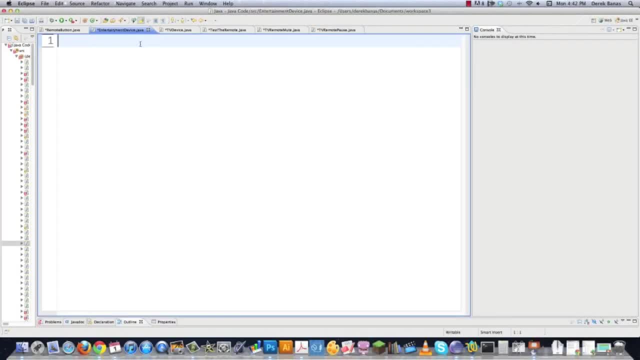 create here is entertainment device, and this is going to be the abstract class, is going to represent every single device that we're going to be creating abstract class entertainment device. And sometimes this is created as an interface, but I never thought it really made that much sense that way. So this is the way that I normally implement these things. So I'm going to say device. 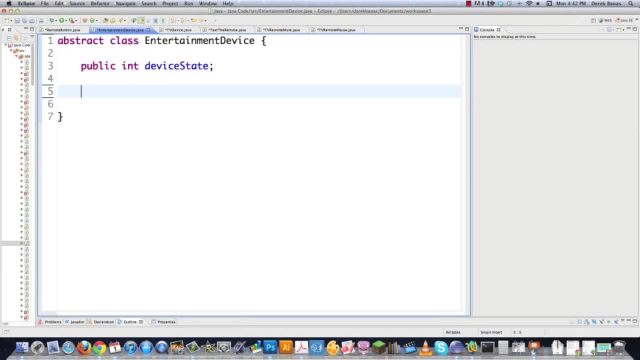 state and all of the code is available underneath of the video in a link. So if you want to check that out- and we're going to define some different fields inside of this- that every single television as well as remote that comes thereafter is going to have And mainly device state is going to either. 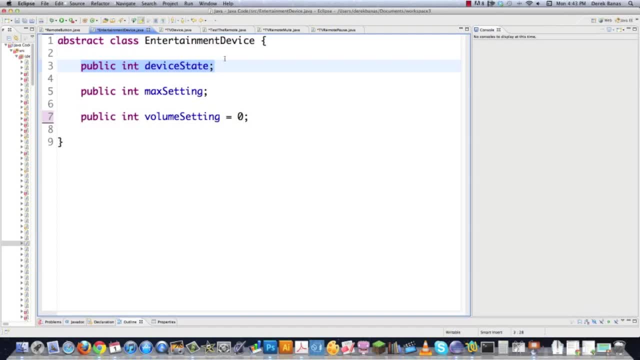 be the current channel that the device is on, or the current chapter if we're using a DVD, And then it's going to be the maximum channel number possible, or the maximum chapter, and then volume settings just going to represent volume settings, All right. So now that we got that all set up, we're 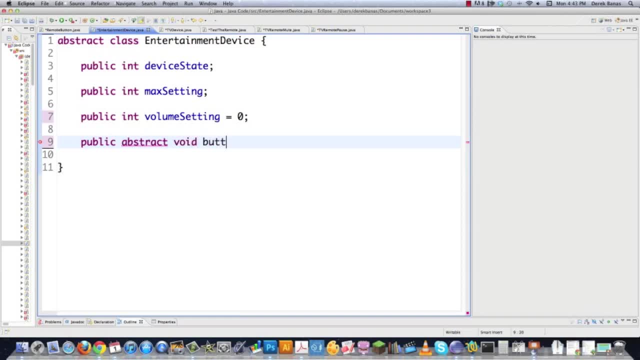 going to define those methods, those abstract methods that are going to need to be defined. So we're going to say, well, what is going to happen when button five is press in, the concrete class that follows is going to have to implement that, And what happens whenever button six is going to. 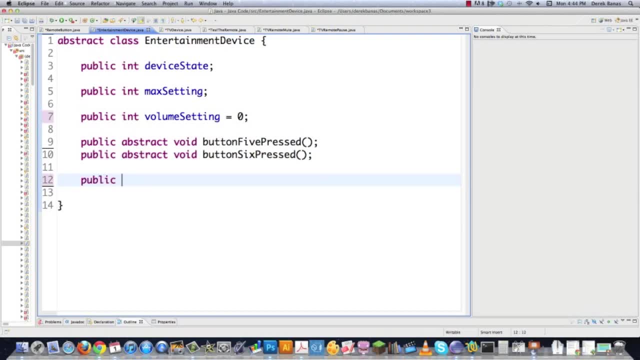 be pressed. Then, on top of that, just to show that everything is going to be working, we're going to come in here and create device feedback, And all this is ultimately going to do is spit out information in regards to the current channel that we're going to be on And we're just going to come. 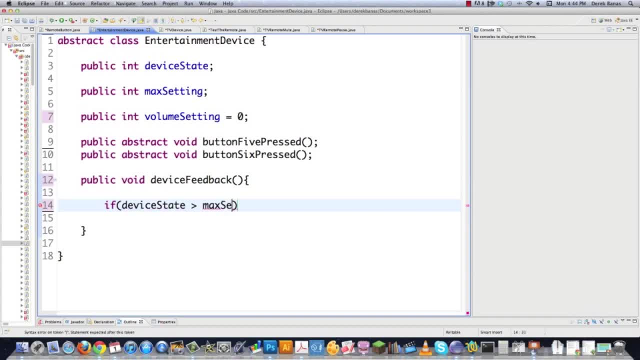 in here and go device state. if it's greater than max setting or device state less than zero- And remember, the device state represents either the current channel or the current chapter- We're going to set the device state or the channel or chapter back to zero. So that's what we're doing. 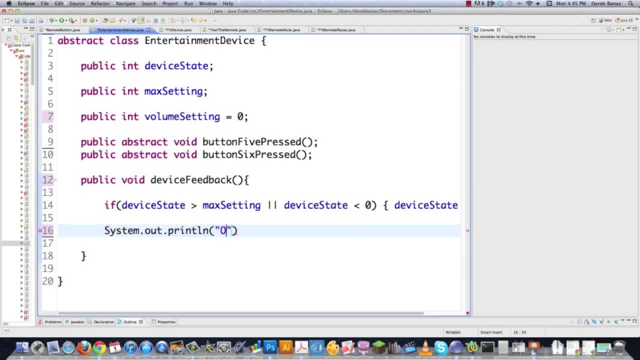 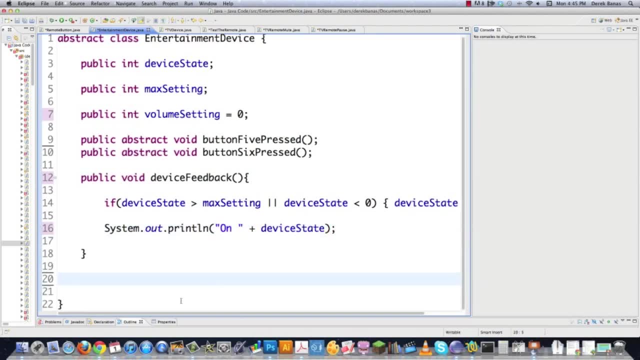 with that guy And then we're going to print out a message and we're just going to say on device state and that's going to shoot out either the channel or the chapter. And then, remember, we said that every single television is going to have a volume. So we're going to come in here and go public void. 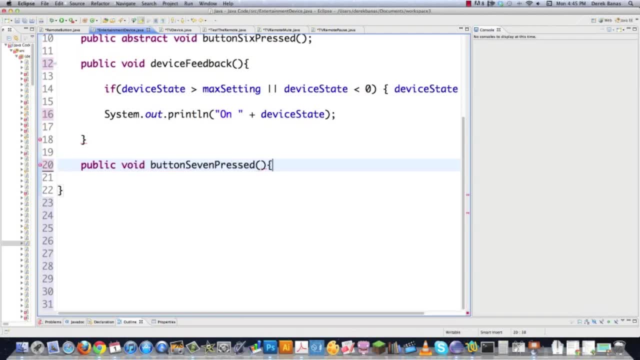 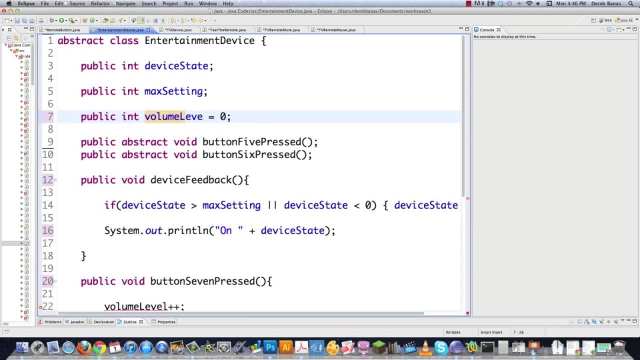 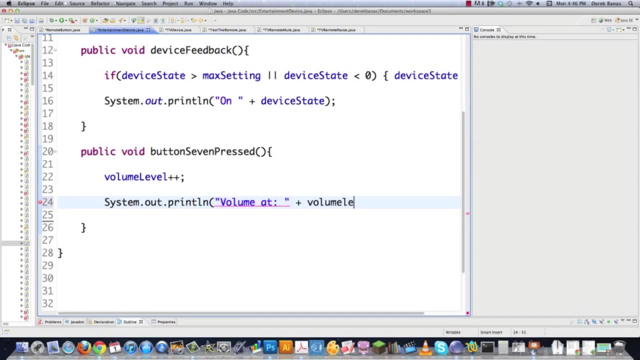 button seven pressed And that is going to represent the volume being increased. So we're going to go volume level plus plus and jump up here and change this to level- because I like that better, Improving this a little bit- And then we're going to come down here and type in volume at and volume level, And there you go. So 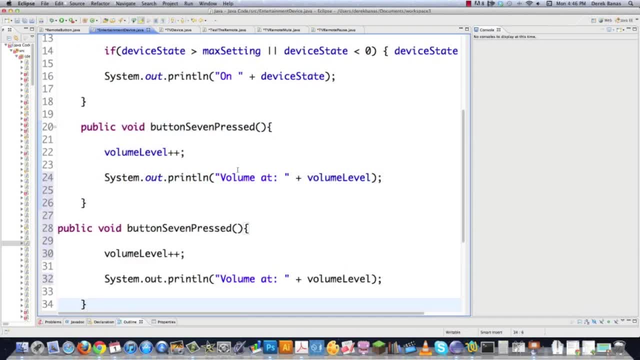 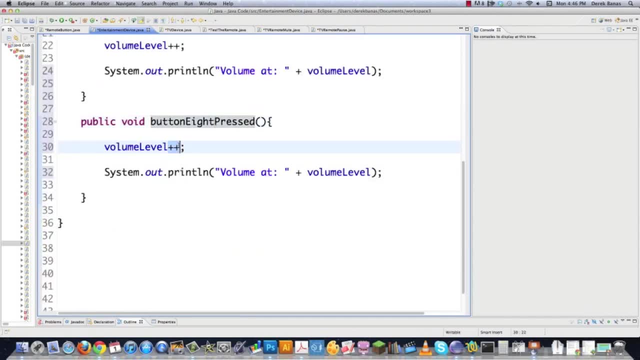 there we are. We're setting just those buttons, because everything that comes afterwards is going to have a capability of raising or lowering the volume, And then button eight is going to decrease the volume, And we're just going to leave that exactly that way. So that is our abstract class. 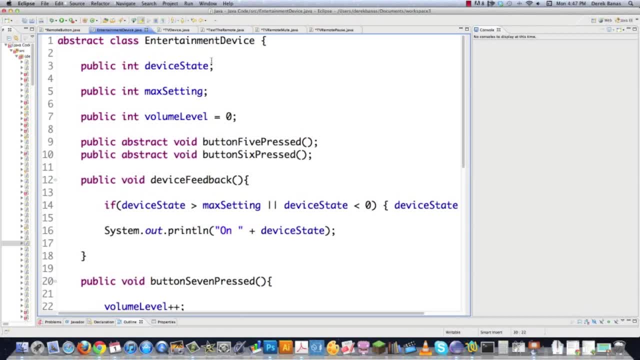 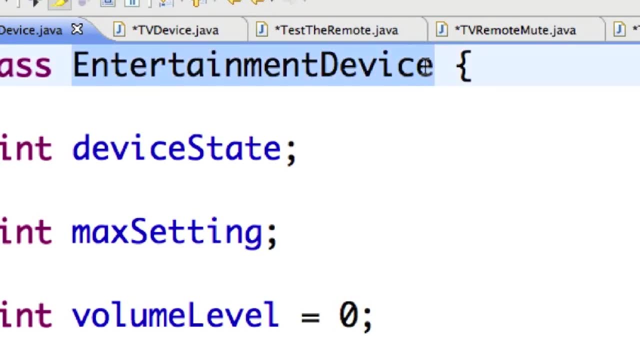 that we're creating, called entertainment device, which every single device will be based off of. So now let's go into TV device And let's actually create one of these guys going to copy this and jump in a TV device, All right, So now we're in this and this is called the concrete implementer, while entertainment device is. 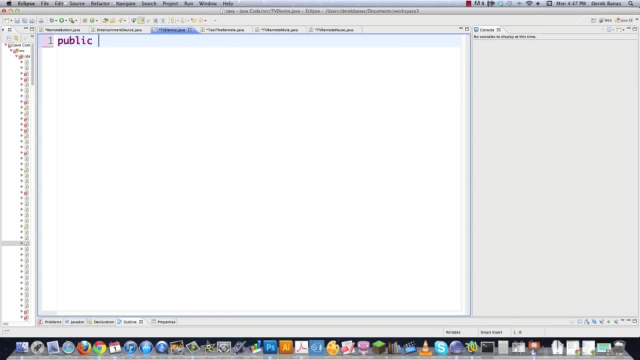 represented just as the implementer And we're going to go public. That's just jargon, by the way, Public TV device extends entertainment device. Then we're going to come up here to TV device and we're going to say, OK, we want to implement on implemented methods, So click on that. There we are. 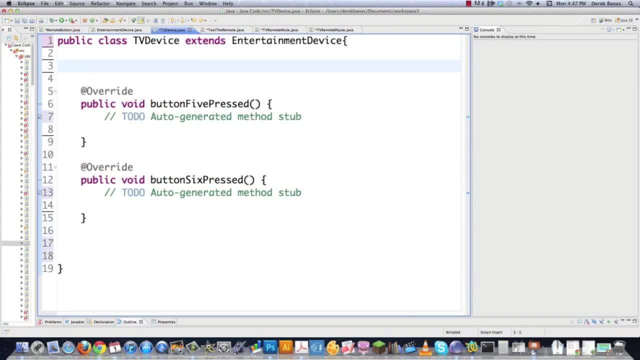 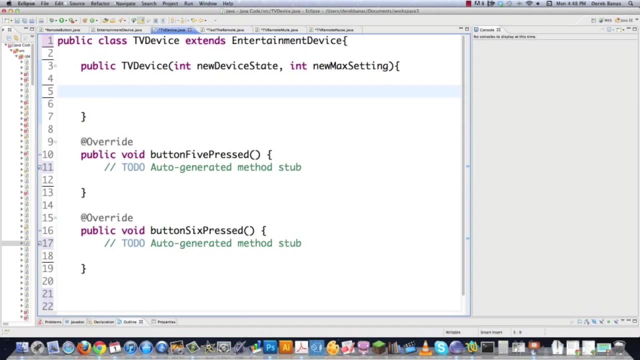 And now we've got all those in there. But then on top of that we're going to create a structure for this public TV device: int. new device state and int. new max setting. So that's all. the different devices are going to have different device states or maximum settings, whether it's 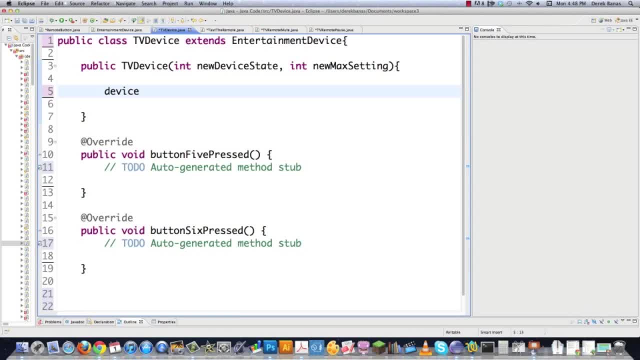 channel or chapter if it's a DVD, And then we're going to go device state which is represented back in the superclass device state, like that, And then max setting is going to be equal to a new max setting. And there we are. So we have that all defined. 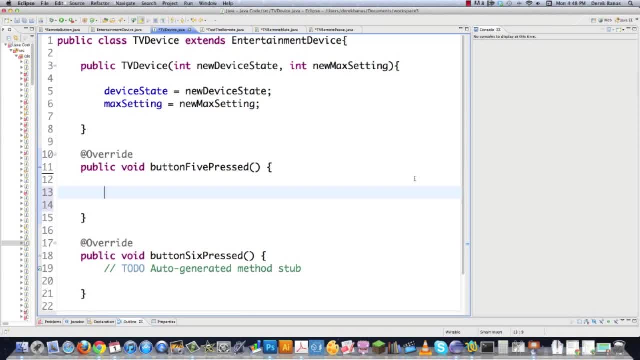 So then we just go into TV device and we're going to go public TV device and we're going to go channel up. So we just have to come in here and talk about how TV is going to be different from the DVD. So out print line, channel down, So that's perfect. Copy that And whenever button six is going to be. 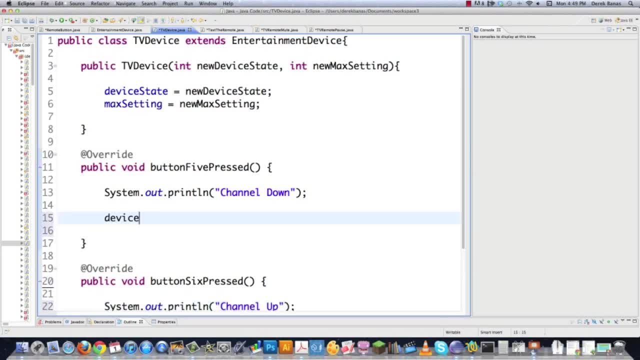 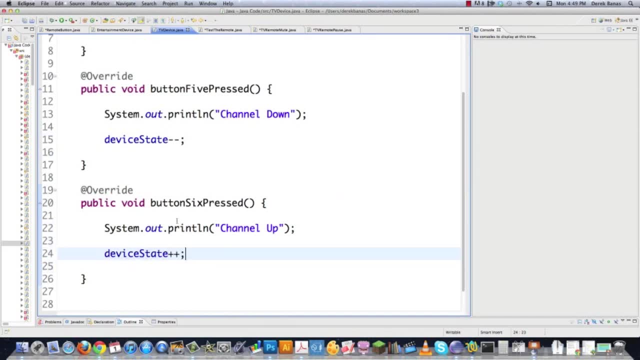 pressed, we're going to say channel up And then I'm going to go device state minus, minus and device state plus, plus And I'm not going to worry about the DVD part that is going to extend entertainment device. If you want to see what that code looks like, you can look underneath the video. But I'm 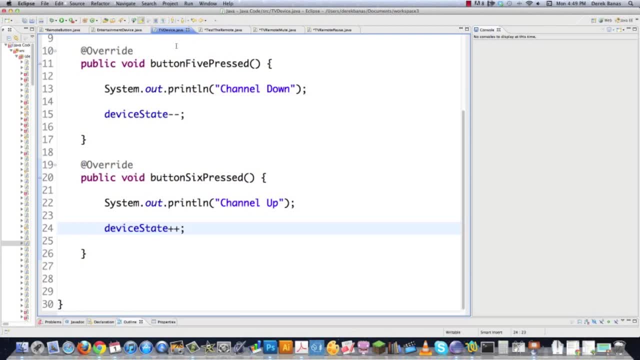 mainly going to focus on the DVD part, And then I'm going to go device state minus, minus and device and then the different ones between the TV's that are going to be created and then the remote controls that are going to follow there after. So then we need to come in here then and create our abstract remote, And I'm going to call that 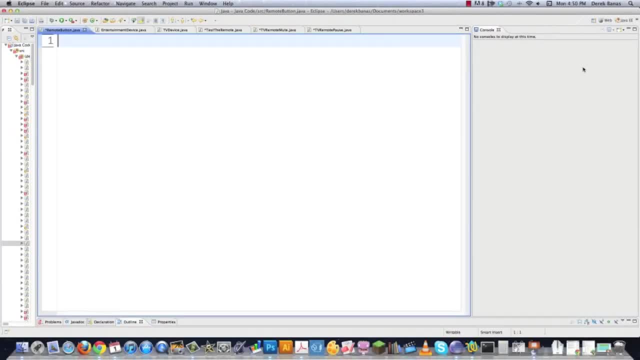 remote button, Javascript on that, And this is called the abstraction layer And it's going to represent numerous different ways we can use this remote to work with all the different types of devices. So I guess your homework would be to go in there and take a look at how the DVD would be. 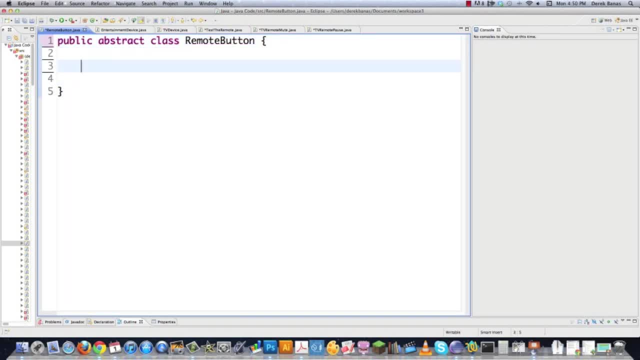 represented here. So another abstract class here. And then we're going to need a reference to the generic device using composition And I'm going to label this as private entertainment device And I'm just going to call it the device like that. 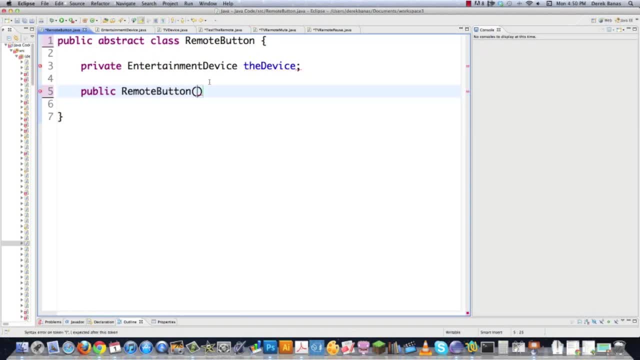 And I'm going to create a constructor remote button And it's going to be passed one of the entertainment devices And I'm going to call it new device. Then just go. the device that's inside of this guy is going to be equal to the new device that's passed over to it. 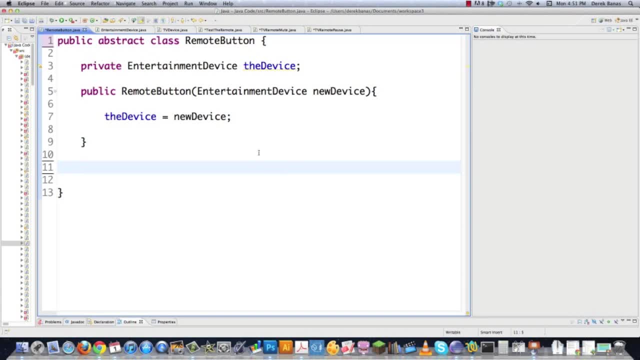 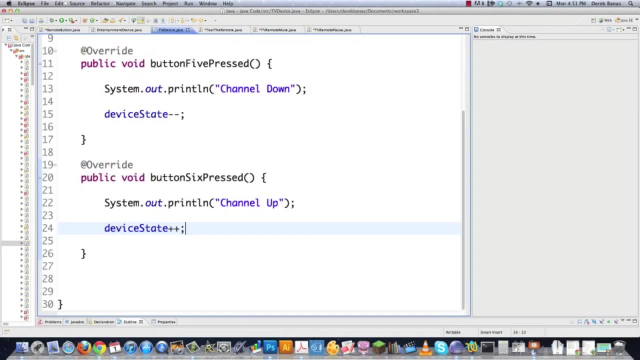 Got all that set up, Then we're going to come in here and reference all of the different methods that were defined for each of the devices. So if you go back into TV device you see here button five pressed as well as button six was pressed. 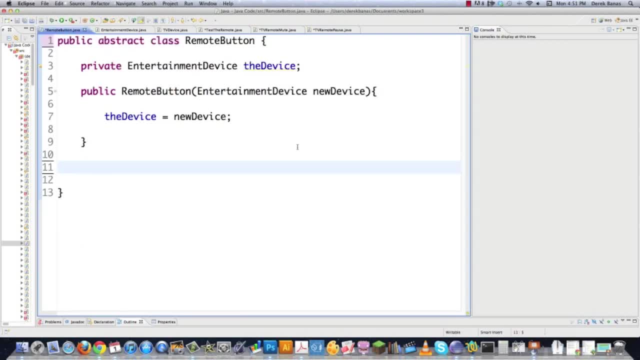 So let's jump back over into remote button And let's define those guys. So we're just going to go public void button five pressed And we're going to go the device And we're going to just call button five pressed inside of it. 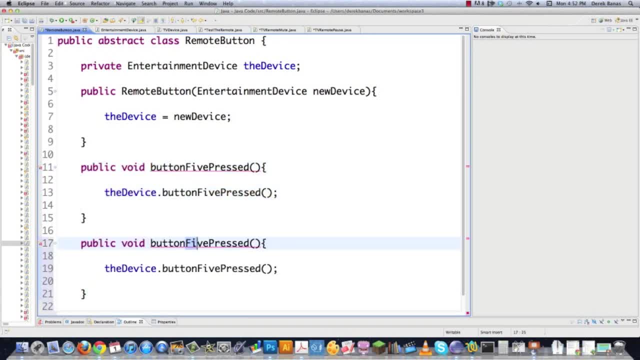 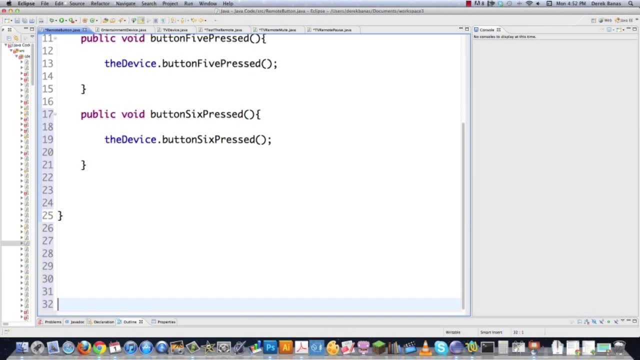 So that's how we're bridging that, And then we're also going to reference button six being pressed right like that, And then if we want to also implement device feedback, which is going to either spit out the chapter number or the channel number that is currently set for the device, 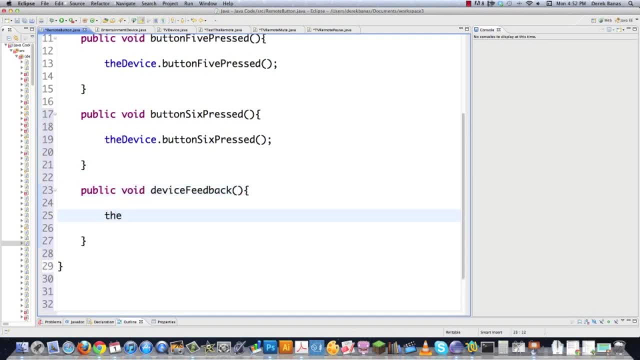 we're just going to go device feedback, like that, And then just go the device and call device feedback And then what we need to do- because this is an abstract class- is define all of the things that those remotes that are going to implement. 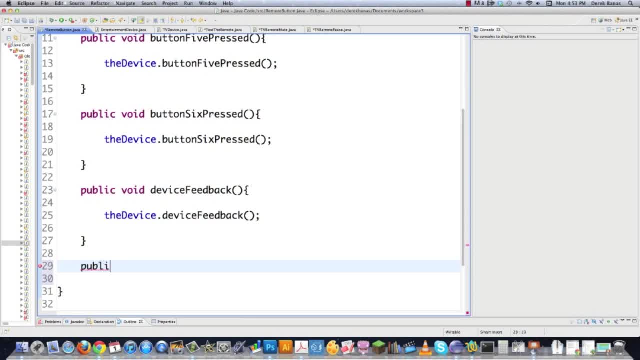 this abstract class are going to need to use or extend anyway. So we're going to go public abstract void. We're going to say that each one of them needs to define what happens when button nine is pressed. And there you did. you just did that. 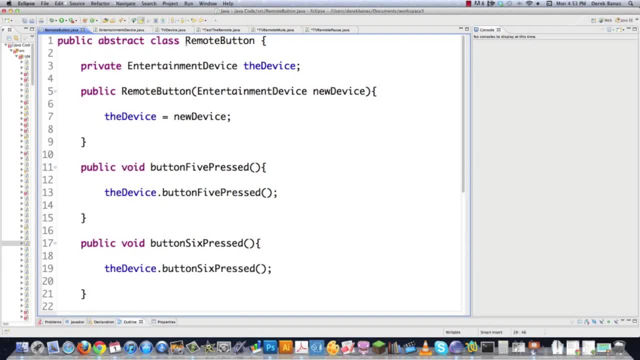 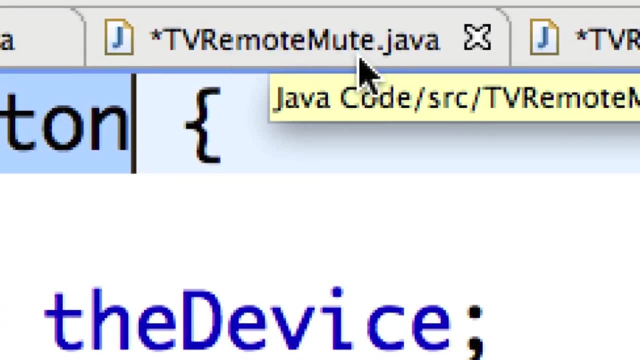 So now we're going to go in and actually create the individual remotes. So we're going to need remote button, which is the generic abstract remote, And then first thing I'm going to do is the TV remote that, whenever nine is pressed, is going to mute everything. 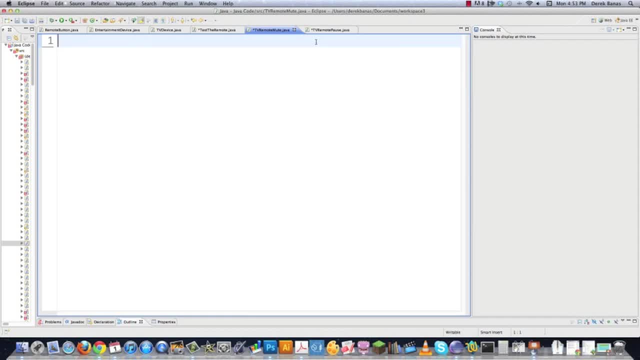 So let's create this And this is called the refined abstraction. Again, there's some jargon for you And we're going to go public class, TV remote, mute, extends, And there's that abstract class. And then this guy is going to say: hey, you need to implement a couple methods here. 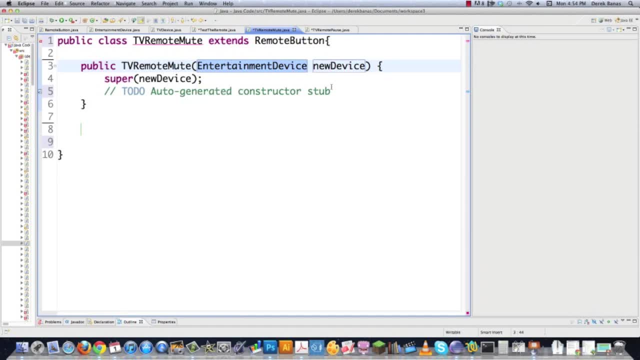 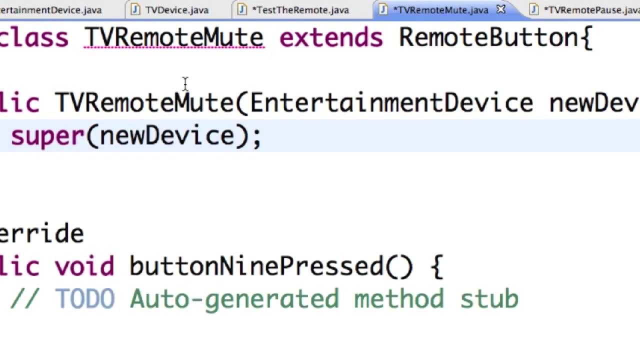 And there they are. There's a constructor we're going to need to set- And basically we don't need to do anything for that, Just get rid of it altogether- And then we're also going to need to implement another method, And that is what happens when button nine is pressed. 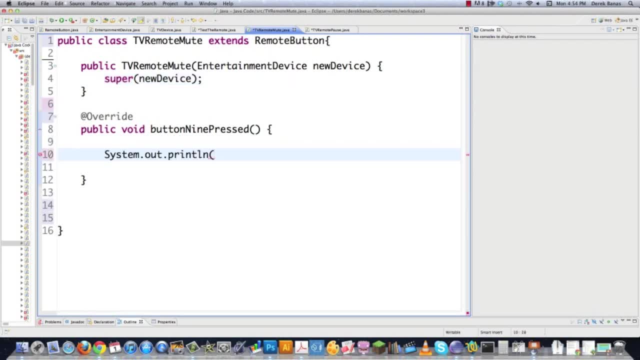 And real. simply, we're going to come in here like that And we're going to print out a different message on the screen And it is going to be: TV was muted. So just different layers of functionality, Everything abstracted out and everything can be changed without affecting absolutely anything else. 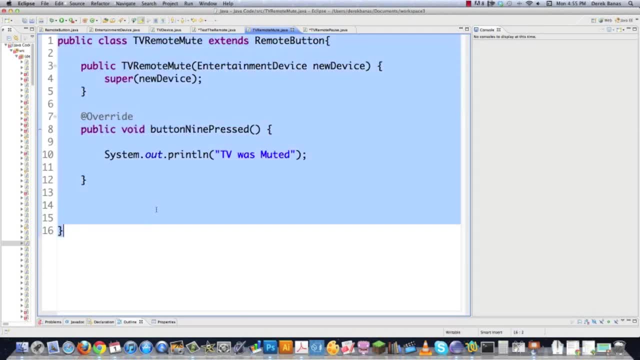 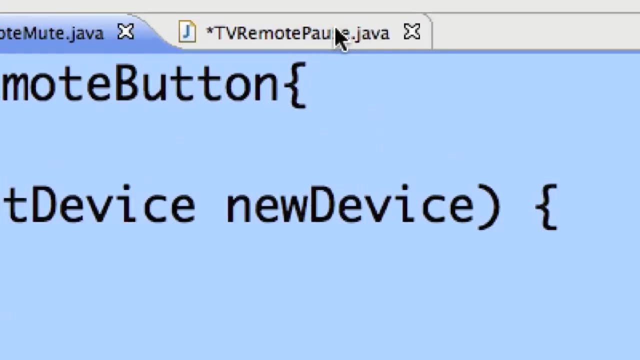 And there you are. Now we're going to come in here and implement the other version of our remote that is going to pause the screen whenever the button nine is pressed, And we're going to call that guy TV remote pause dot Java. Paste that in here. 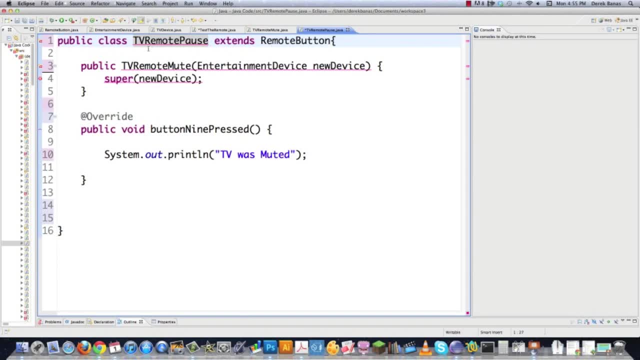 Remote pause extends remote button. Everything's going to be the same there And this is going to be pause Again. everything else can stay the same. And then TV was paused. OK, Now we go into test the remote to see that everything is working. 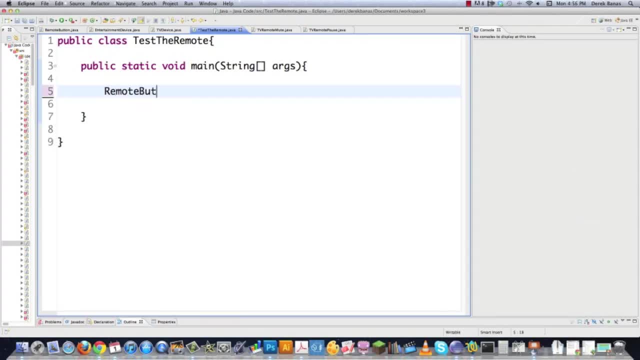 So we're in test the remote And I'm going to go remote button. Again, I'm going to be referring with an abstract class here And I'm going to call this the TV And then go new TV remote mute. And right here I'm going to go new TV device. 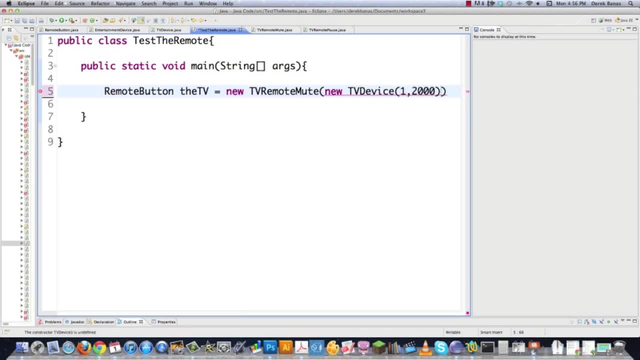 See, this allows me to use multiple different types of devices, not even just the TV devices, If you wanted to implement a DVD or whatever, But it's tons of functionality. And then we're going to create another one. I'm going to call this the TV two. 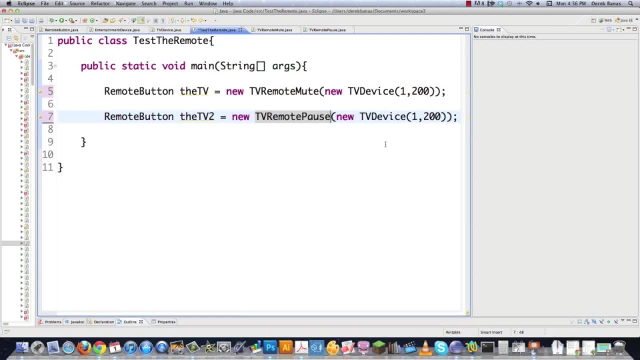 And then just call this pause, like that. And it's also going to create another television And just so you can see what it would be like if you would want to create a DVD. It's going to operate much the same way, So I'm going to go remote button again. 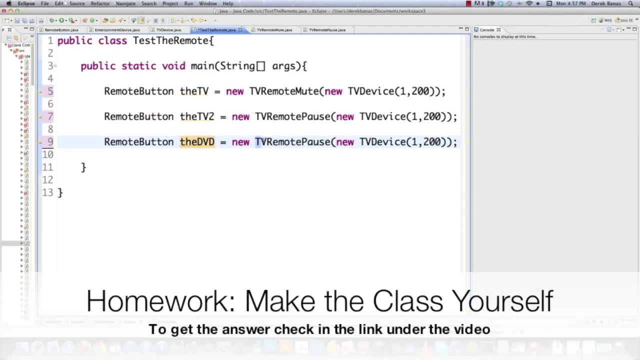 Except this would be called DVD. And this is then I'd have to create a different remote DVD remote like that, Instead of creating Remote pause and so forth, And then I'd have to go in here and go DVD device. And then let's say, our DVD that we create has 14 chapters. 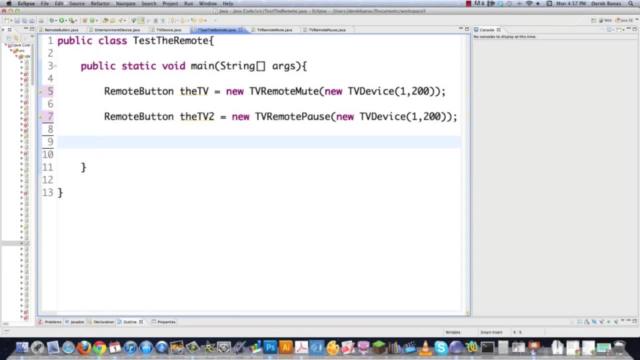 Anyway, the code's underneath the video. if you want to play around with that- And you should- if you want to completely understand the way this guy works, Okay, so now let's go in here, Go system out And check this guy out. 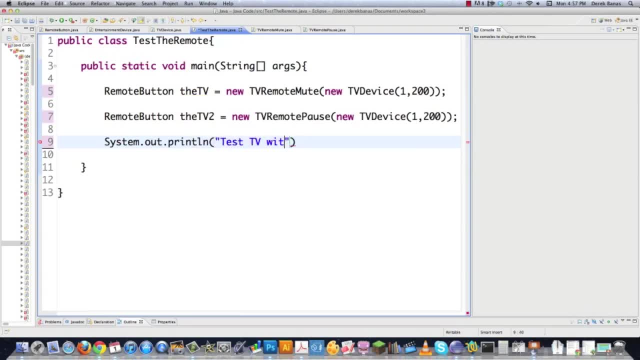 So first thing we're going to do is test TV with mute. That's the first test we're going to do, And then we're going to go the TV And we're going to say button, You can just see right here, Five is pressed. 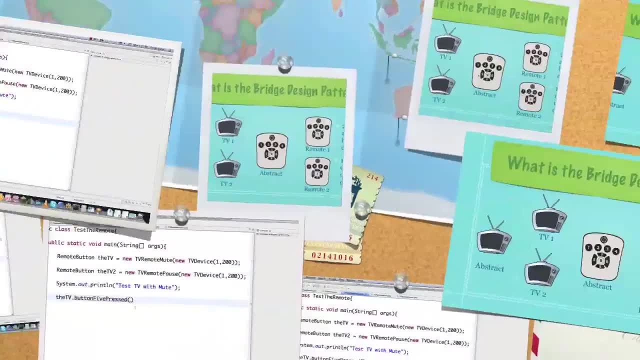 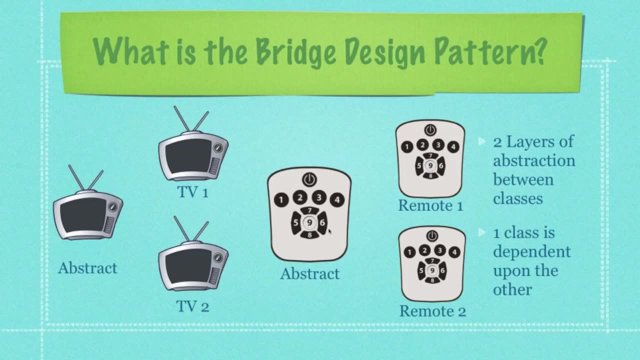 Just click on that What's going to happen when button five is pressed, And you can see right here: Button five is going to make the channel go downwards And button six is going to make it go up. And just so, if you don't remember, 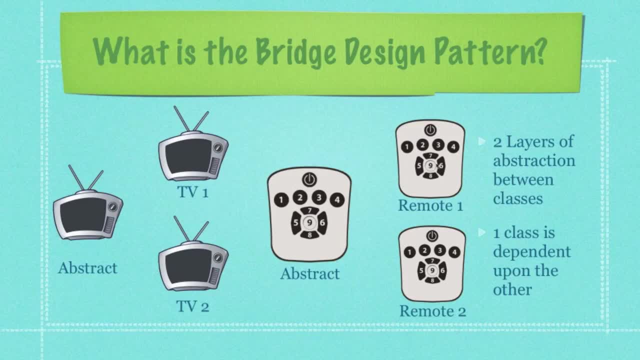 The remote that is going to change nine into mute is right there, And then this one right here is going to pause live television as if it's in ADVR. Okay, hopefully that makes sense. If you have any questions, leave them down below. 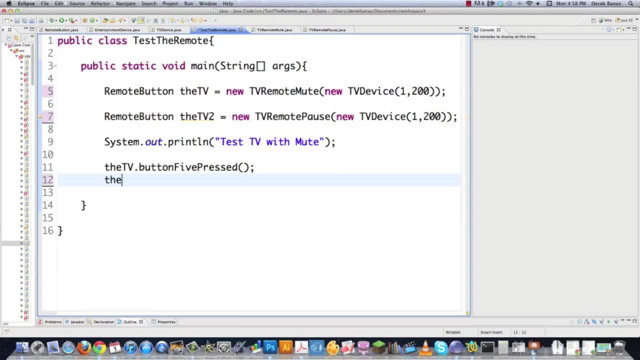 Okay, so this is the TV that has mute, And we could also go the TV And then go button six pressed And there's that, And then we can go the TV button. Now, this is the one that's going to change. 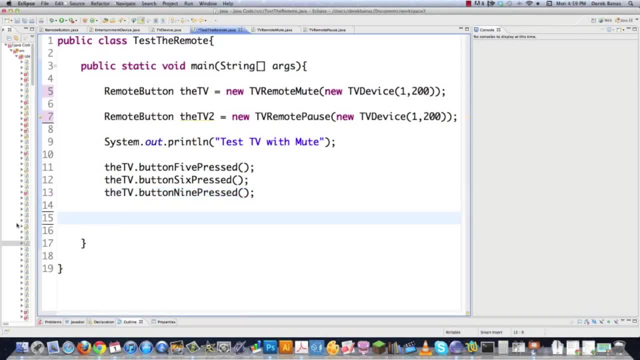 Button nine has been pressed. And there you go. And now we're going to be able to look at the difference. So let's go and copy this guy, And this time we're going to perform a check for the test TV with pause. 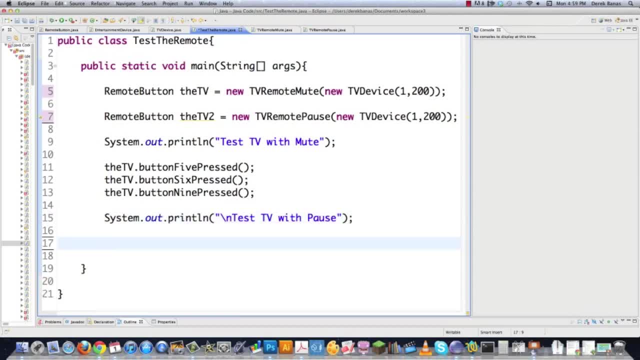 And how it's going to differ from the TV that has the mute. So we're going to go the TV two And then we're going to go button five pressed. There's button five, And then, if we would just want to do something a little bit different, 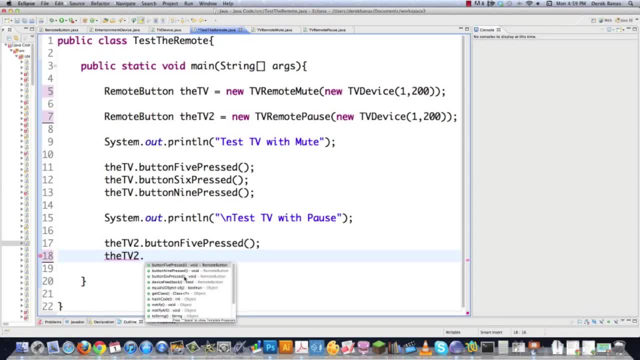 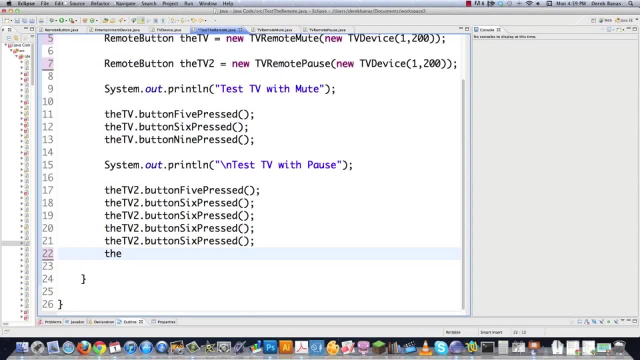 The TV two And let's say we want to do button six pressed, Which is going to make the channel go up, And let's have the channel go up multiple different times- Okay, so there's like four times- And then to also provide or cover what happens when button nine is pressed on this. 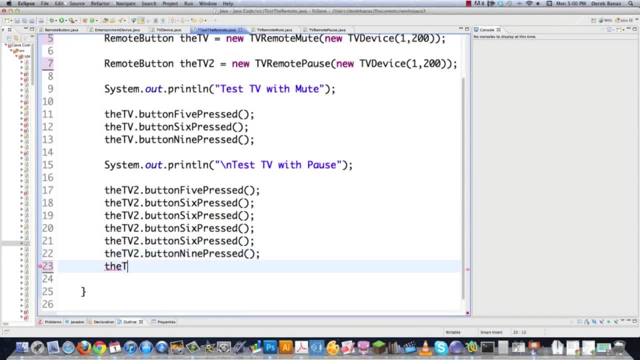 There's that, And then on top of that, if we want to get feedback on exactly what channel we're currently on, Device feedback, Of course, is the only option there I'll save. So let's execute it and see what happens, And there you can see. 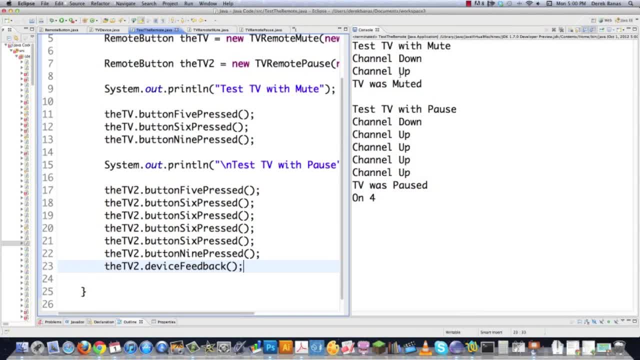 Here's the TV remote that is specific to the device. That has the capability to mute everything, And here you can see channel down, Channel up, And then whenever nine's pressed, TV was muted, And you can see likewise TV was paused whenever button nine was pressed here.